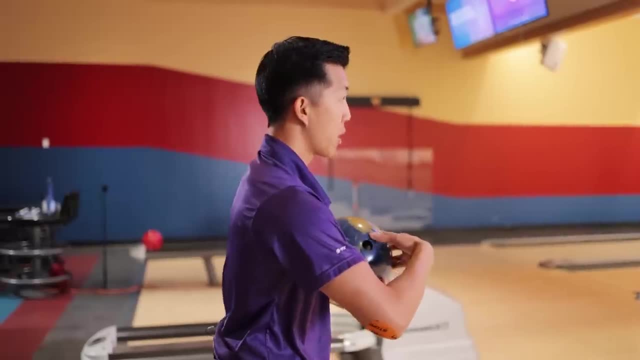 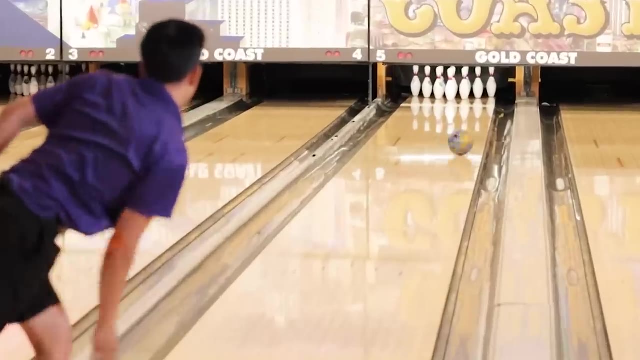 move around the lane, feel it out, figure out where you need to be, And obviously you want to pick the option that lets you hit the pocket the most time. So we're going to move a little bit to the left. Now it looks like we might have moved a little too far. 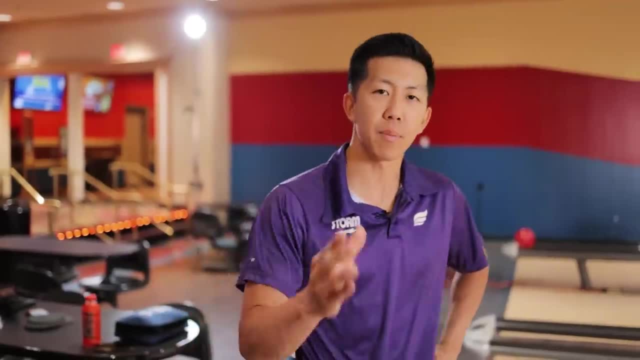 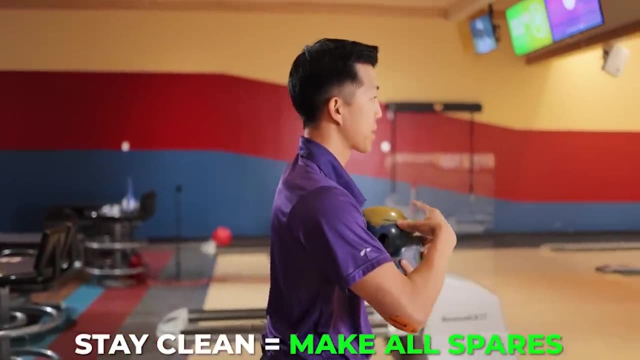 but here we finally found the pocket. A little light in the pocket, but as long as we can keep hitting that one three, we're going to be able to give ourselves the best chance to score 200.. Now remember, the goal is to throw a double and stay clean. Anything more than a double is going. 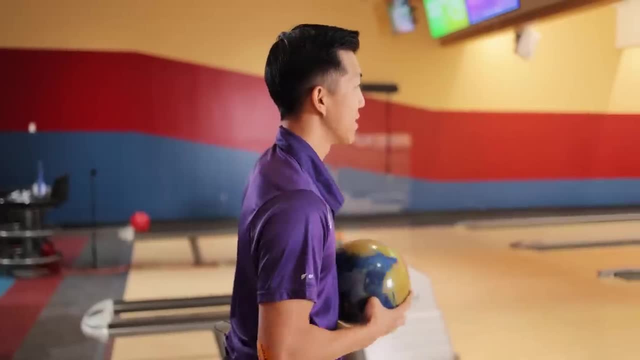 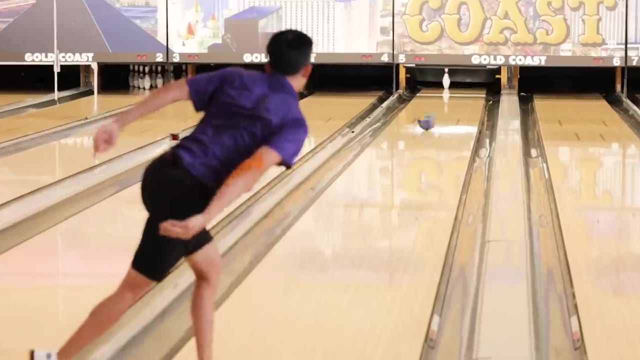 to be a big bonus, but that doesn't necessarily mean we want to start getting lazy and start missing spares, So we really need to dial in on our second shots. So far, so good. We're clean, We've got a strike and a spare Again. 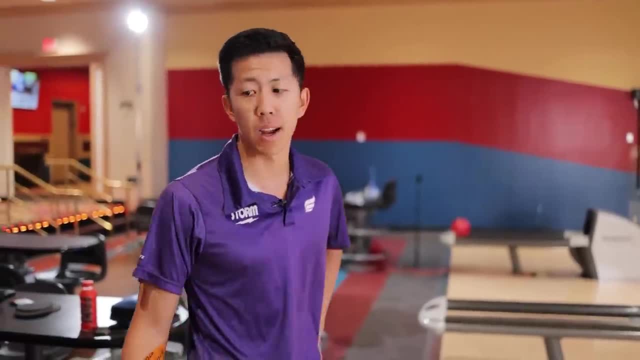 we're still looking for that double, So we're going to keep it really simple. We're in the one three now Probably don't want to move a whole lot. If you're just getting started with bowling, these micromanaging moves probably are not something you want to think about, Just keep. 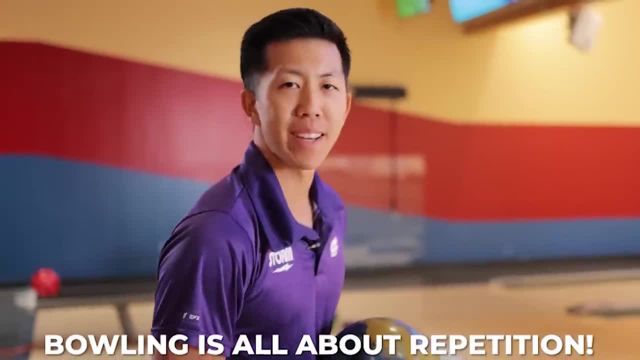 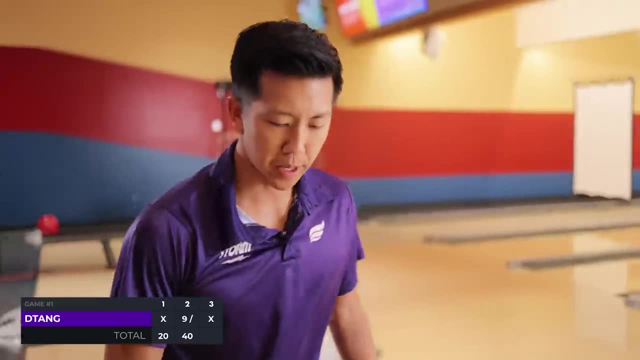 it simple: Try your best to make good shots. Put yourself in the right spot. Do the same thing every time. I just made another shot. We're not thinking too much, We're just trying to hit the one three Task at hand The most. 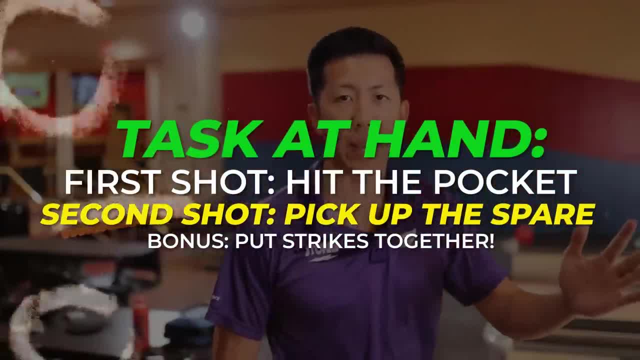 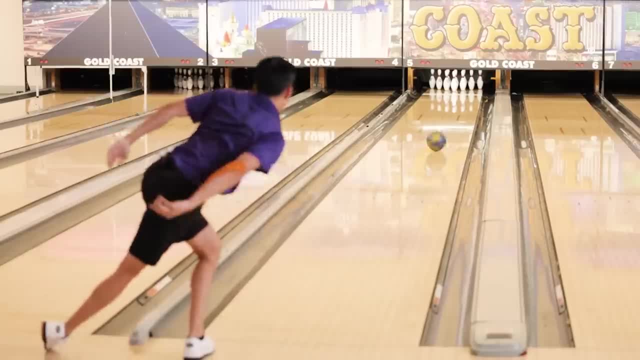 important thing you need to focus on is the task at hand. First shot: hit the pocket. After that, pick up the spare. All right, here we go. We're going to try again. Try our best to hit the pocket once more. All right, we hit the pocket once more, and now we have our double. Now we just have to. 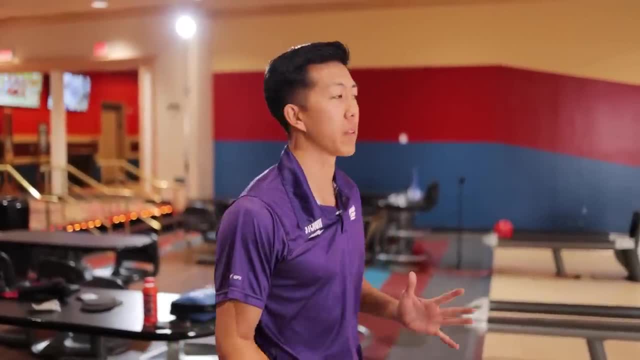 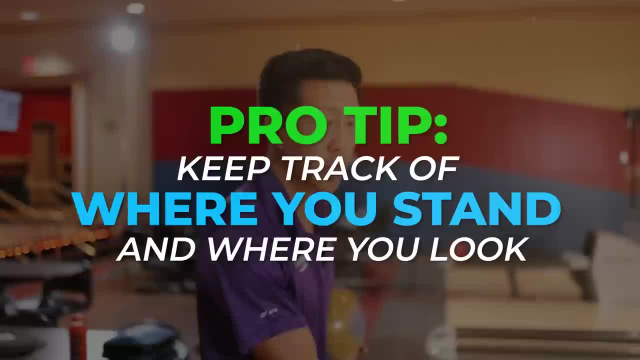 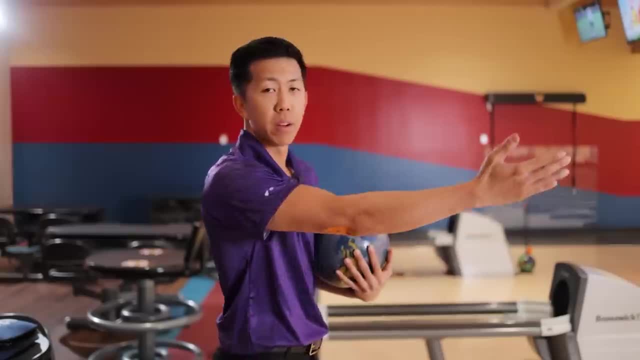 we need to do. A really important thing to remember is keep track of where you're standing, keep track of where you're looking. The more specific you can make it, the higher chance you're going to have of hitting the same thing over and over again. There are seven arrows on. 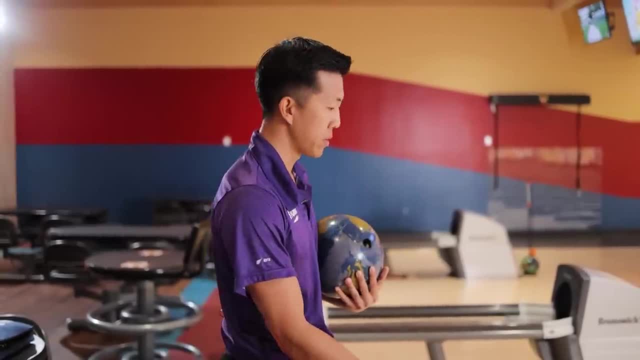 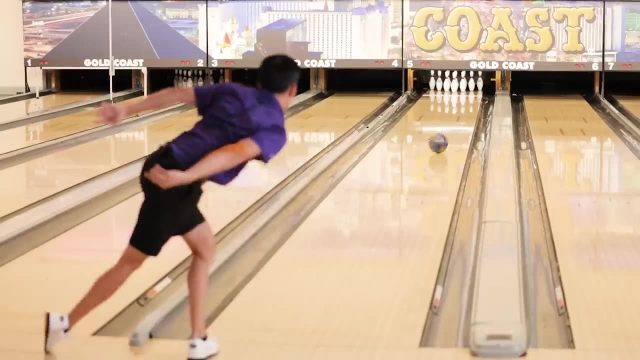 the plane. There are sometimes five, sometimes seven dots on the approach. You want to try your best to stand on the same one every time. Here we go, We're going to try to hit the pocket once more. So I threw that one a little too far to the right and it overhooked. So going back to the Brooklyn, 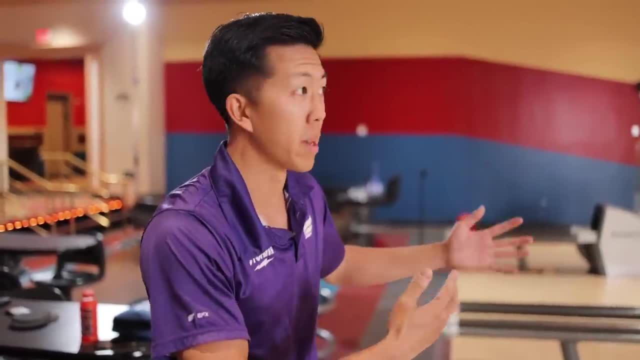 if we kind of did the same thing and we just tried to throw it to the right, it could have overhooked even more. We might have missed the head pin, We missed the pocket. What do we do now? A lot of people might start to freak out: Oh my God, I missed. Now there's more pressure. We 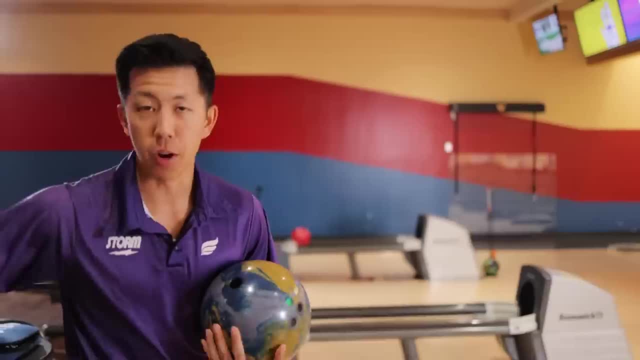 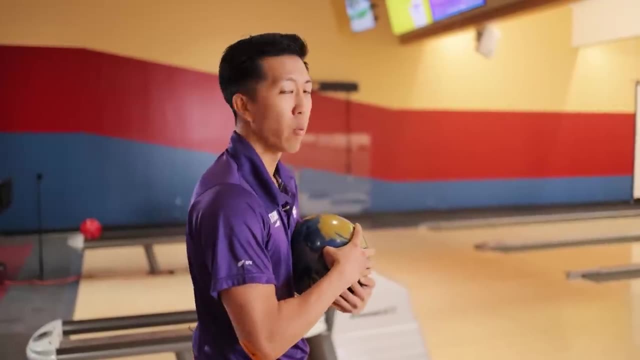 talked about the task at hand before. We just got to focus on picking up the spare. now, Don't get frustrated. There's a lot of people who are a little more on the result-oriented side, so when they don't get what they want, they get mad, and that just gets things out of whack for the next. 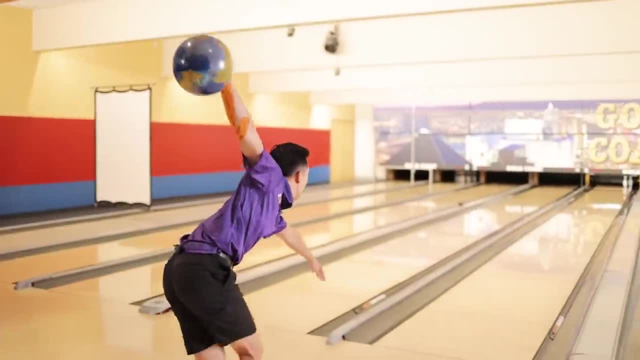 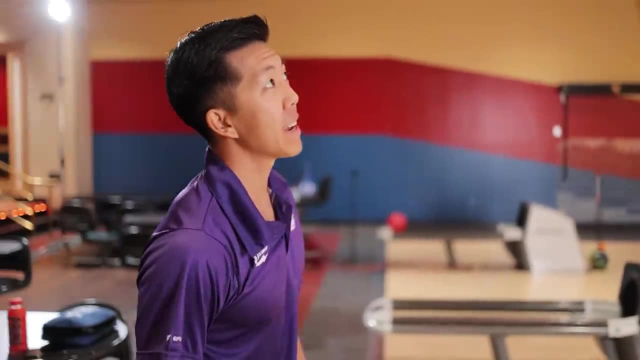 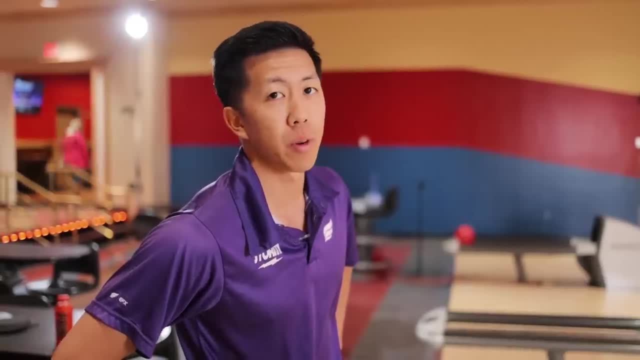 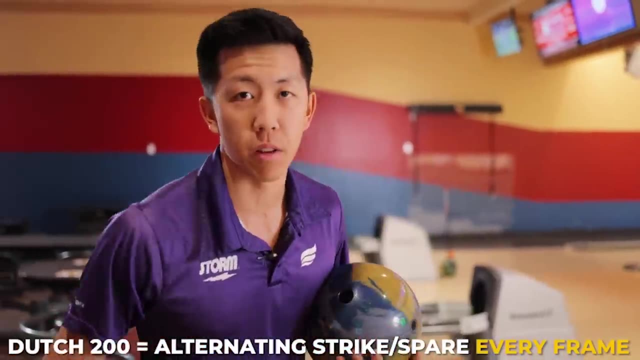 200. A nine spare. every frame gets us there. I believe- and I know there's going to be people in the comment section- that say you don't have to throw a double to shoot 200.. What about the Dutch 200?? That is true. That is the one instance where you do not need to throw a double to shoot. 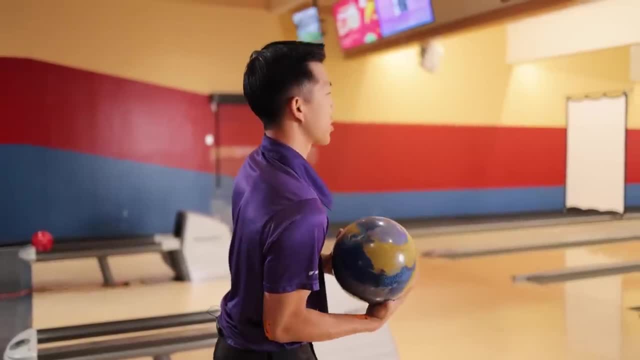 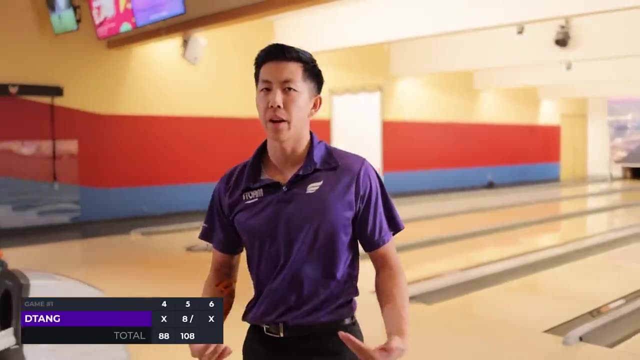 200.. So we're just going to try to make a better shot. We're not going to overthink it. Let's just try to make a good shot. Now, there is a decent amount of luck involved. You are somewhat in control of that luck. You know that one wasn't a good one. We're going to try to make a better shot. 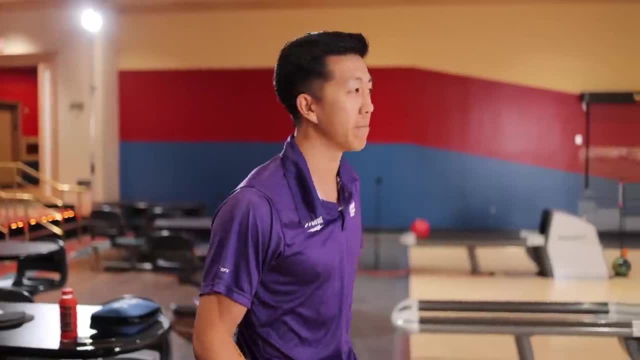 The prettiest strike. We got pretty lucky there. You know, if you do the right things, you get lucky. Figuring out how to do the right thing to get luckier- it's going to be in another video. Here we go. We're just going to keep trying to hit the pocket. Stay nice and clean. 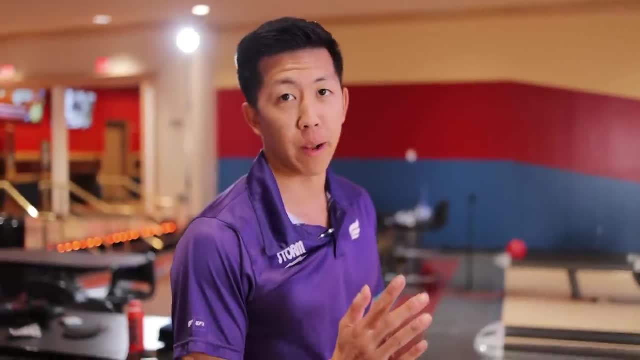 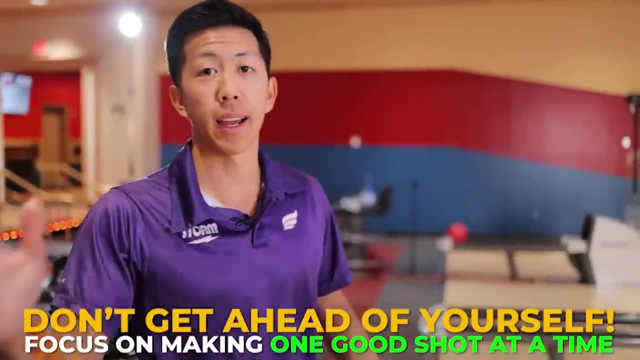 Now we're really looking good. We got two doubles. now We don't want to start thinking about 200 because we're not in the clear yet. We want to think about the task at hand, and I'm going to hammer it home: the task at hand, what's in front of you? because the second, we start looking ahead. 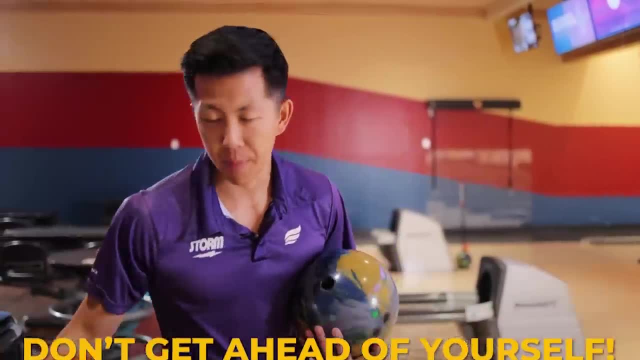 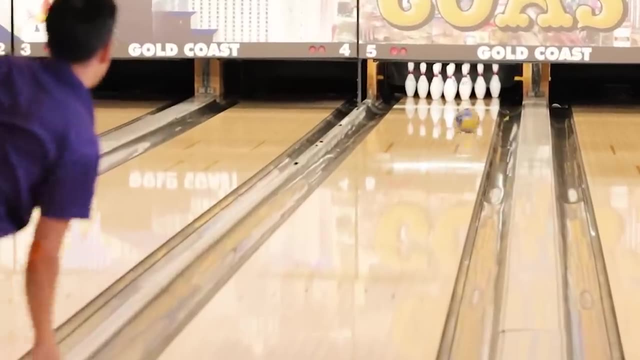 now we're shifting our energy, We're getting distracted and we're not going to be able to make the best shot possible. So let's say I do get a little excited. I start thinking about it a little too much. Now we got to get back on track. What do we do next? We focus on the spare. We don't want to. 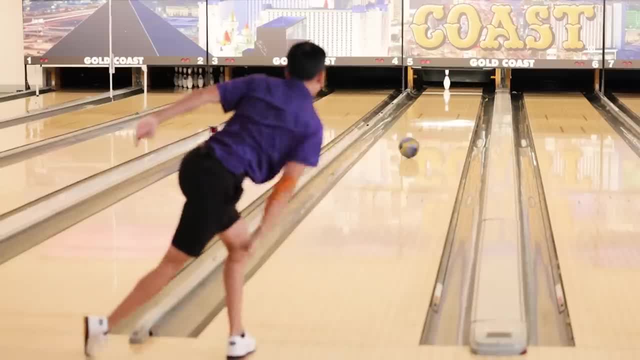 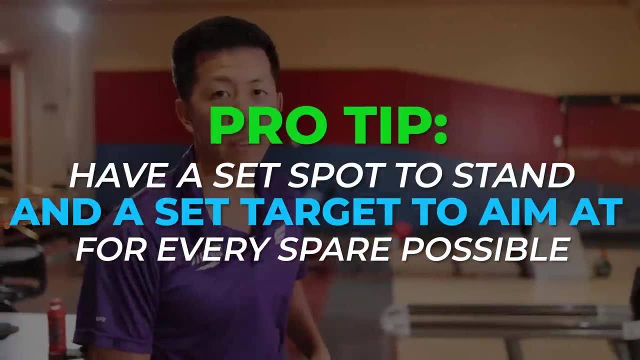 get upset. We just keep moving forward. Simple Single pins, in my opinion, are like free throws. It should be autopilot. Every time you see a single pin, you should have trained yourself to know where to stand, what to do, go up there and execute the shot. If we're not at that point yet, 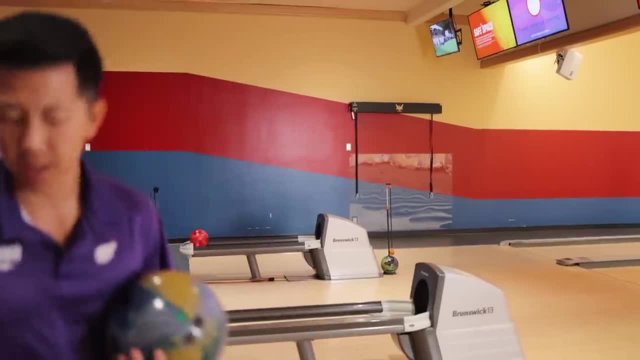 we've got more videos in the future to help. Let's shoot some more spares. Spare shooting is the number one key to shooting 200 consistently and often. So again, we're just going to try to focus on making a good shot. 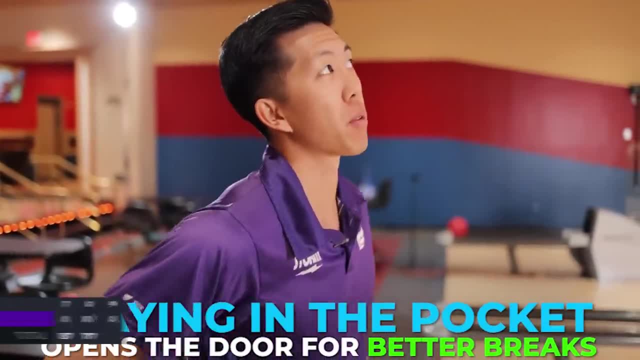 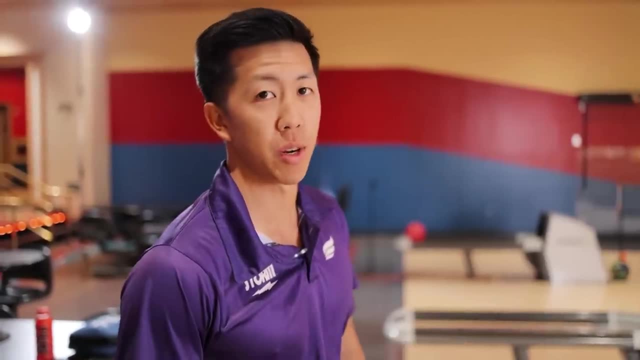 So this is the importance of staying in the pocket. You see, we've only really missed the one-three one time this game and we've set ourselves up perfectly to shoot 200. Now all we have to do is keep it on the lane. If we get seven, we shoot 200.. We're not thinking about. 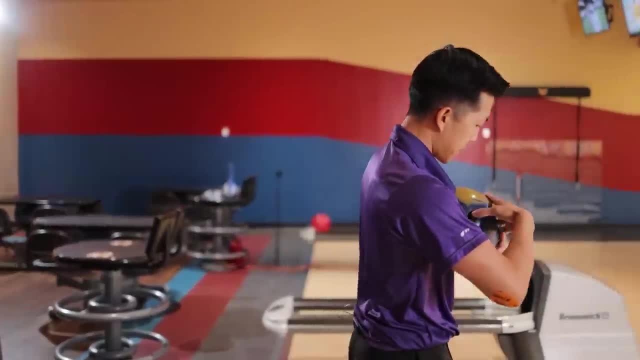 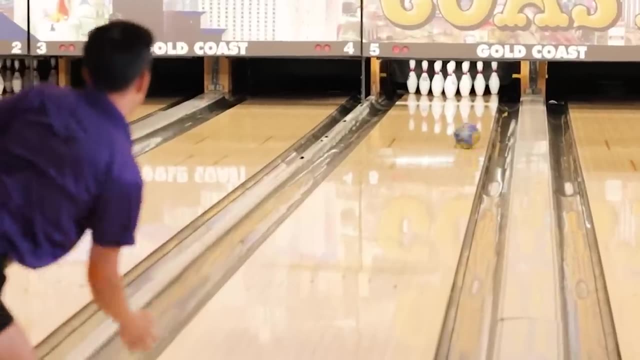 getting seven. We're trying to hit the pocket again, So we're going to get up here and just make the best shot possible. Focus on your target. Don't forget where you're standing. Make a good shot. May not have been the best shot, but we put ourselves in a really good position. 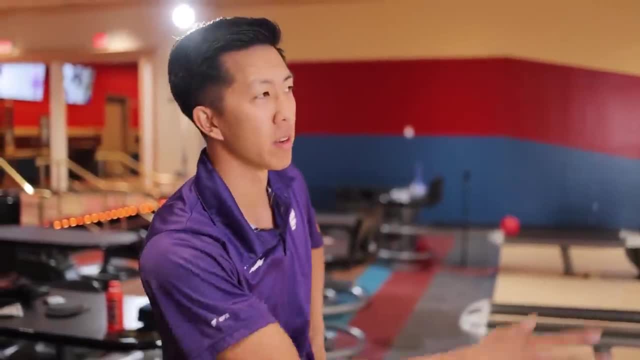 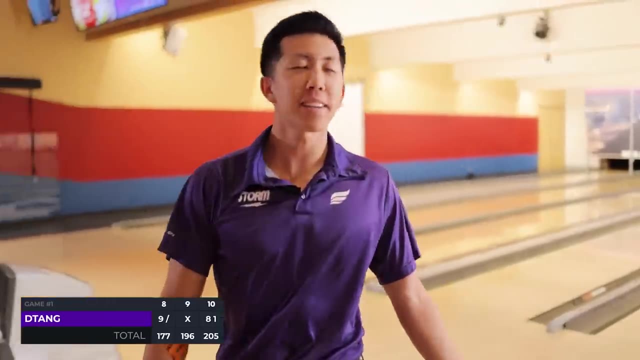 frames one through nine, and now we don't even need the spare. We have 203 on the board without even hitting another pin. Here we got one. It doesn't even matter. Technically, it's not a clean game. So we didn't do everything that we said. but you don't have to just throw a double. 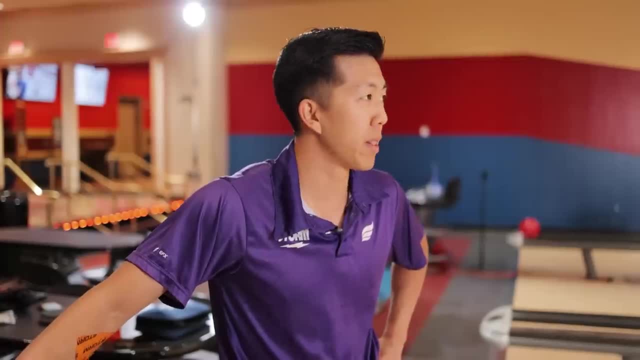 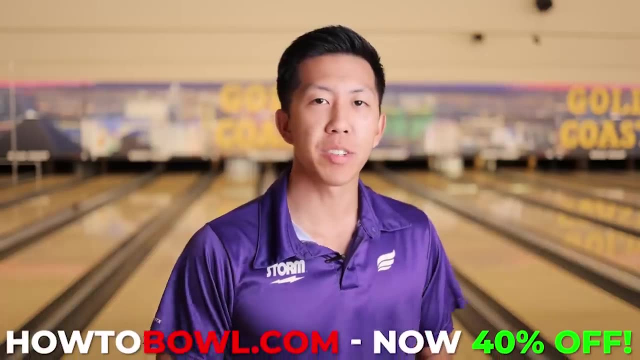 and stay clean and shoot 200. There are a lot of ways to get there, sometimes a little bit of luck. If you get five or six in a row in there, your chances are really good. You got to throw that double. You got to stay clean at the bare minimum. If you guys are interested in videos like this, 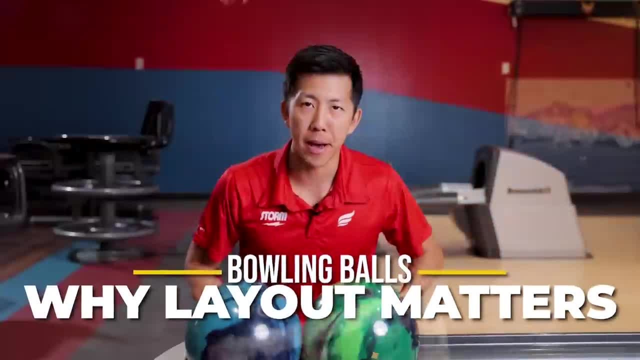 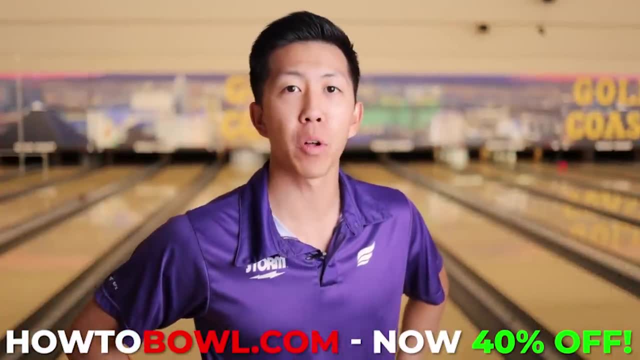 or you want to take your game to the next level, make sure you check out our online bowling course. We have a library full of videos ranging from equipment, physical game improvements, lane play and even tips from other pro bowlers. So if you're interested in becoming the best bowler that you, 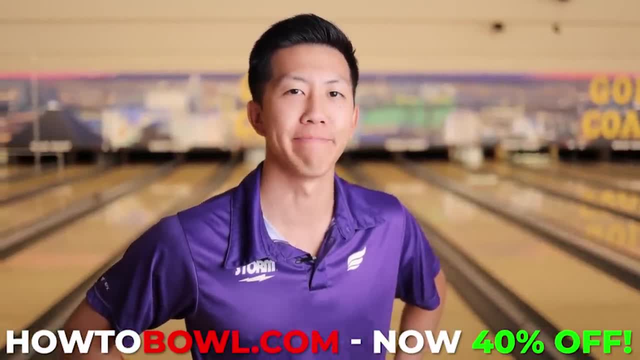 can be check out the link in the description below. Thanks for watching and we'll see you in the next one.